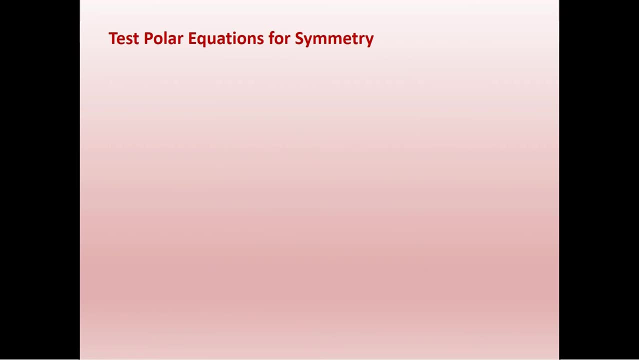 that it has pi over 2-axis symmetry. Now the last one we have is polar symmetry. So this is with respect to the pole, which is basically origin symmetry in rectangular. So notice, if this is theta, that this also has to be theta, which means that this whole thing would be pi plus theta. 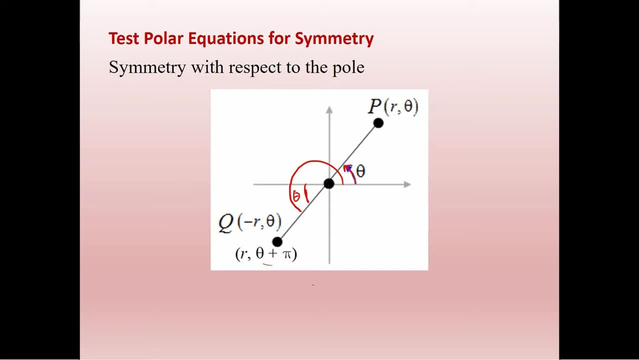 right, So theta plus pi. So what we're going to do is we're going to replace theta with theta plus pi. okay, So if we change theta plus pi or theta into theta plus pi, and we still get r, 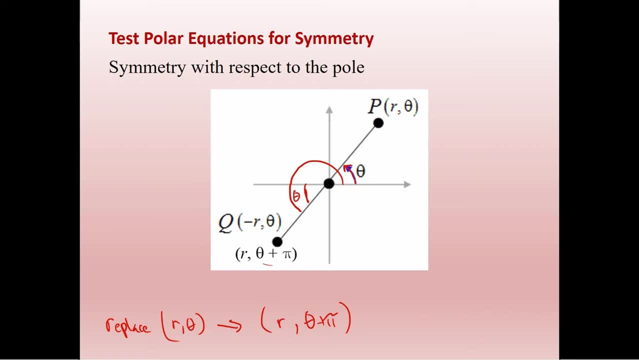 then we know that it has polar symmetry. Another way of doing it would be to replace r with negative r and see if we still get theta out. Generally not as effective a method, but it can still be done. So now a few things that we want to mention. If the substitution doesn't give an 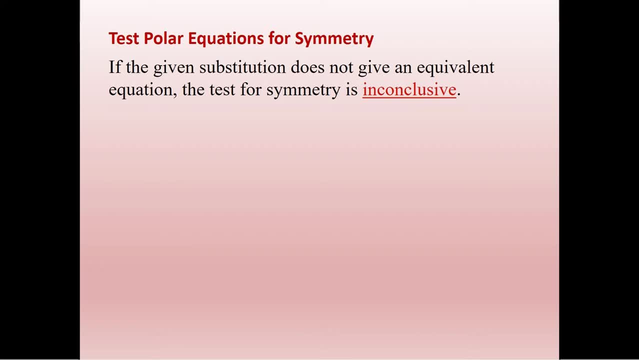 equivalent equation. that does not mean that it does not have symmetry. It's just inconclusive, These tests for polar symmetry. they don't say that it doesn't have symmetry, It just says that it does okay. So if it does work, 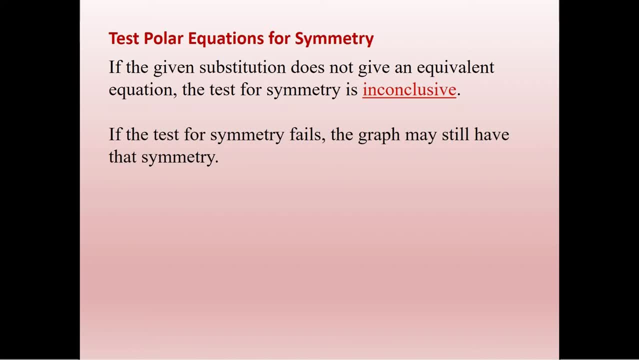 you know it has symmetry. If it doesn't work, it's just inconclusive. and we may still have symmetry, okay. Now, one of the reasons that we do this is because there are infinite number of representations of any given point. We can change r to negative r, change our. 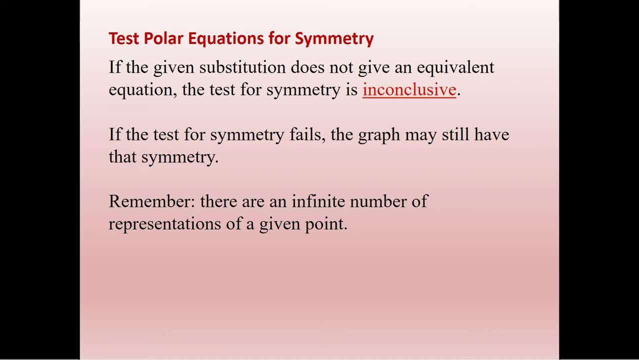 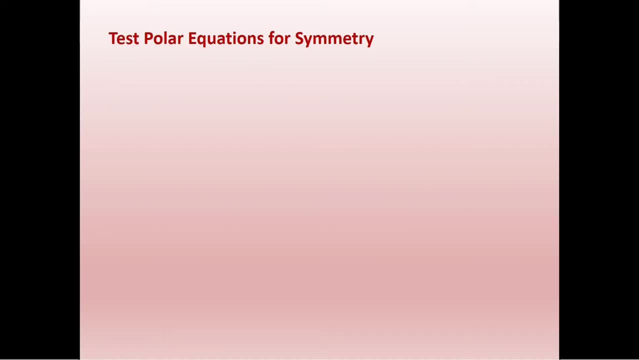 theta into pi plus theta. So because of all of this stuff, we have to say that a failing test of symmetry is just infinite. So if we change r to negative r, we can change our theta into pi plus theta, and we can change r to negative, r to negative r. So if we change r to negative, 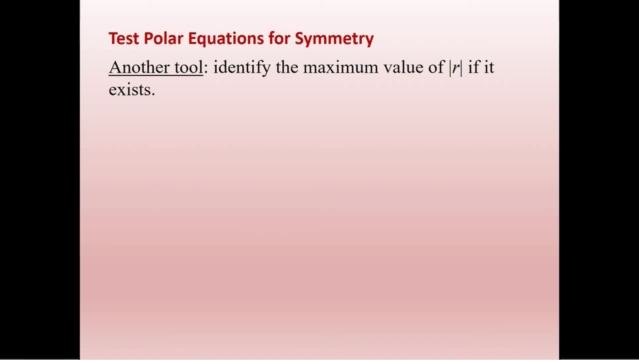 and we change r to negative, we can change r to negative, we can change r to negative, and if we change r to negative, we can change r to negative. so it's just inconclusive, okay. One other tool that we can use to talk about: 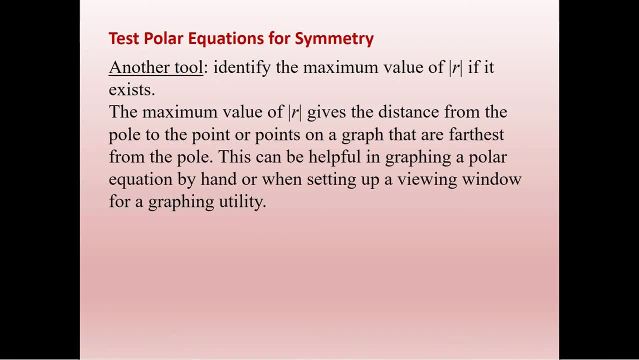 symmetry is if we identify the maximum value of the absolute value of r, which this is basically just gonna be the distance from the pole to the pointer points on the graph that are farthest from the pole. okay, So this can be helpful in graphing polar equations. 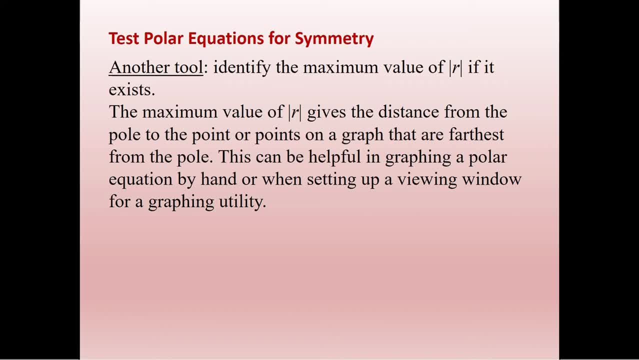 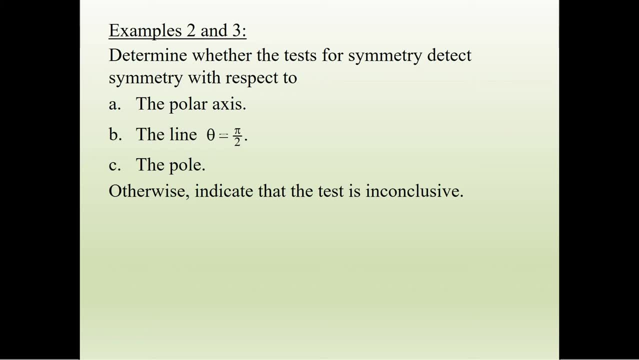 when you're doing it by hand or if you're using a graphing calculator that does polar for setting up the window. okay, So let's look at a couple of examples real quick and we're going to determine whether this actually determine or detect symmetry with respect to the polar axis, which would be like x-axis. 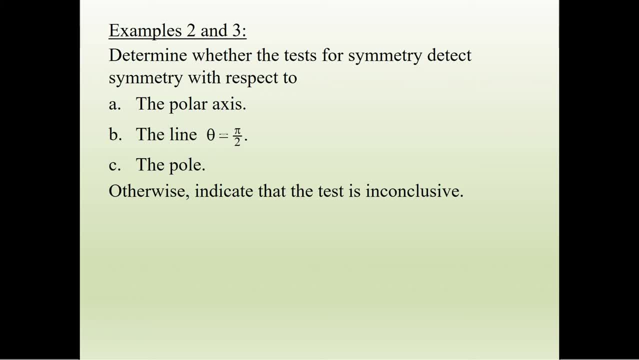 symmetry: the line theta equals pi over 2,, which would look like y-axis symmetry, and the pole, which would look like origin symmetry. okay, So let's start with 8 cosine 2 theta. So let's start by saying, okay, we're going to replace theta with negative theta, So r equals 8 cosine of. 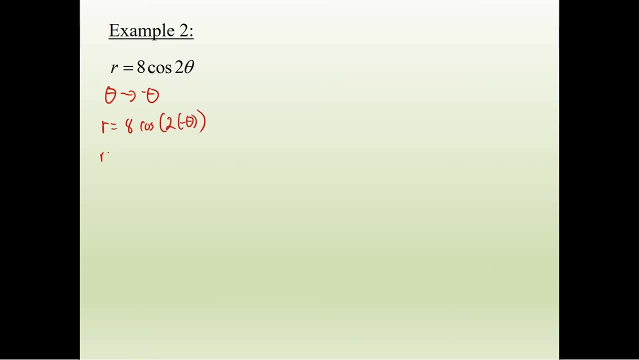 2 times negative theta, which is just r equals 8 cosine of negative 2 theta. but cosine is an even function, so it's going to eat that minus sign. We get r equals 8 cosine 2 theta. Well, that's the same thing we started with right: 8 cosine 2 theta. So yes, this has polar axis symmetry. 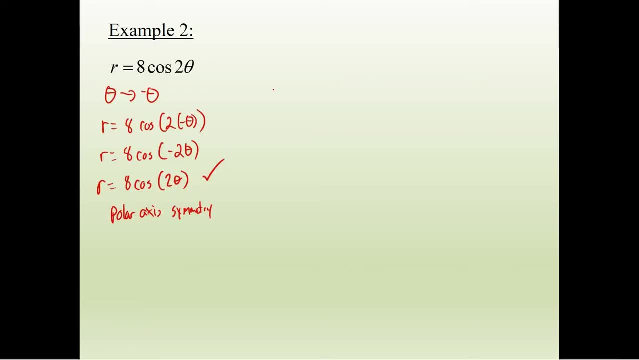 Okay, Oops, sorry. Now we've done polar axis symmetry and we've done 8 cosine 2 theta, So now we're going to get r equals 8 cosine polar axis. let's do pi over 2 symmetry, So in this case we're talking about pi minus theta. 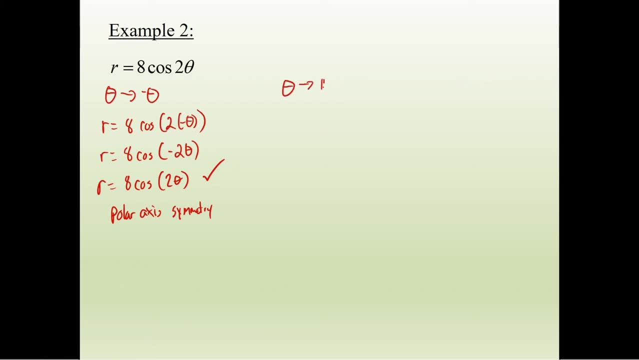 So we're going to substitute theta for pi minus theta. So we get r equals 8 cosine 2 times pi minus theta. So this is just r equals 8 cosine of 2 pi minus 2 theta, But 2 pi minus 2 theta. 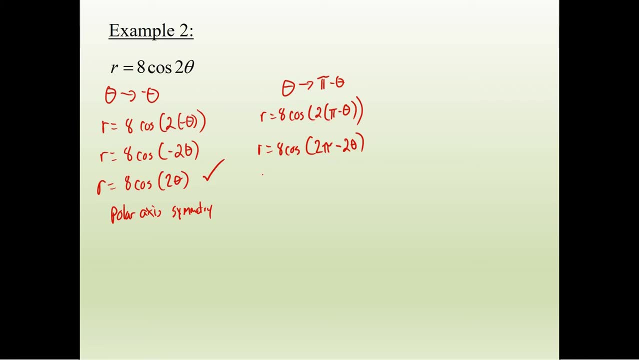 well, this would be the same thing as r equals 8 cosine of negative 2 theta plus 2 pi. Well, remember, because of the periodicity of cosine, r equals 8 cosine of negative 2 pi plus 2 theta. So this would be the same thing as a cosine of negative planeta plus 2 pi. 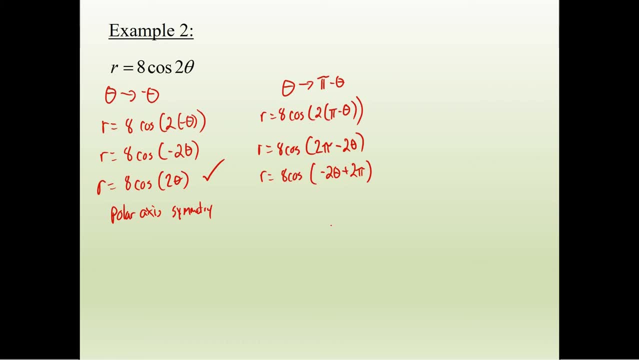 cosine. If we add 2 pi, we just get back to the same place. So we can kind of just ignore the plus 2 pi and just say negative 2 theta, because they're going to be coterminal, right? Plus 2 pi just means a coterminal angle. So since they're coterminal, their cosines are equal. 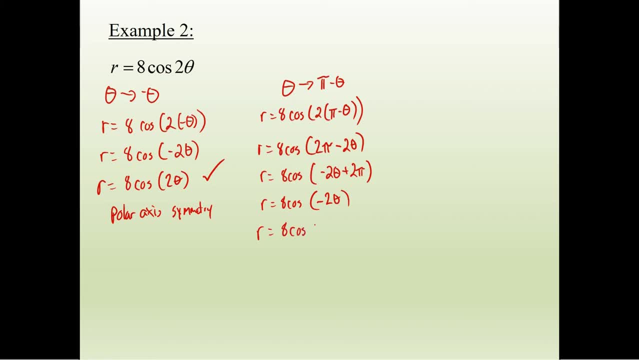 but this is an even function, so it's just going to eat the minus sign and we get back to 8 cosine 2 theta. So it does have pi over 2 symmetry. Now for our last polar symmetry, or pole symmetry. 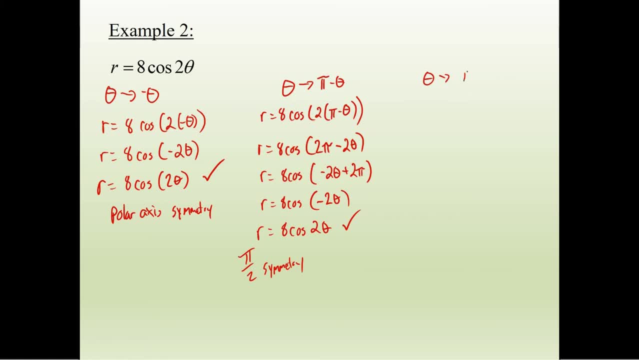 then we know that we're going to substitute theta with pi plus theta. So we get r equals 8 cosine of 2 times pi plus theta. so we get r equals 8 cosine of 2 pi plus 2 theta. but once again that's just the. 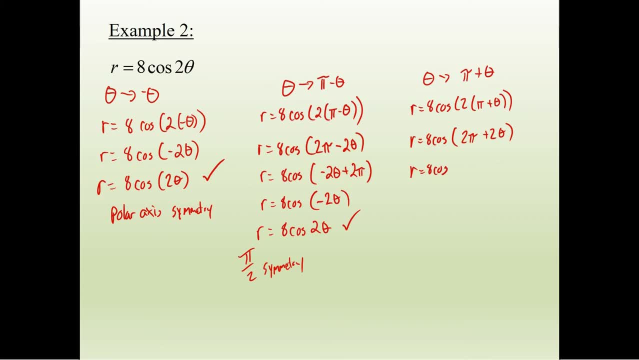 excuse me, the periodicity, the periodicness of cosine. if we add 2 pi, that's just a coterminal angle, so we can ignore the plus 2 pi and just say 2 theta and bam, this has pole symmetry. so we know that 8 cosine, 2 theta is actually going to have symmetry across all of those things. 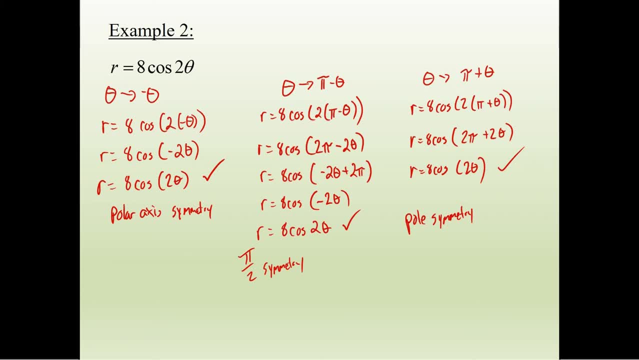 and since we haven't really talked about it yet, we you could graph this, of course, on any graphing utility or a website, and you'd see that it's actually a flower or a rose that looks like this and has symmetry across this line, across this line and across this line. 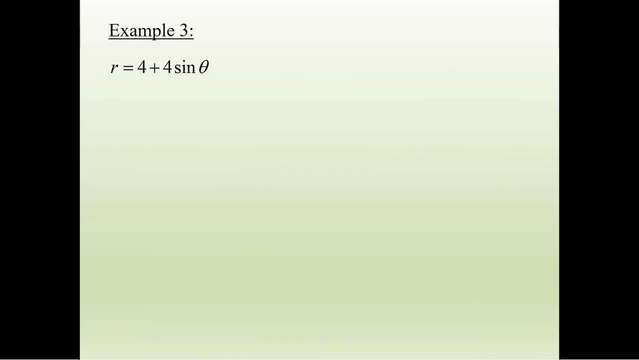 all right, 4 plus 4 sine theta. so now we're talking about an odd function with sine. so if we plug in that, we get r equals 4 plus 4 sine negative theta, but the negative theta just comes out as a negative sign, since sine is odd. 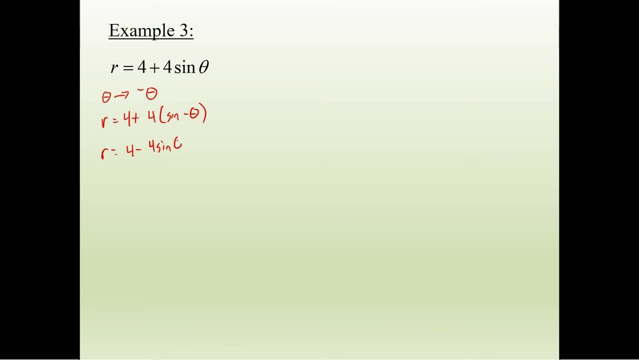 we pull the minus sign out, you get 4 minus 4 sine theta, not the same, so inconclusive on the polar axis. if we do pi minus theta, then we get r equals 4 plus 4 sine of pi minus theta. but here I don't have any, you know, periodic rule or some rule that lets us, uh, easily cancel that out. So